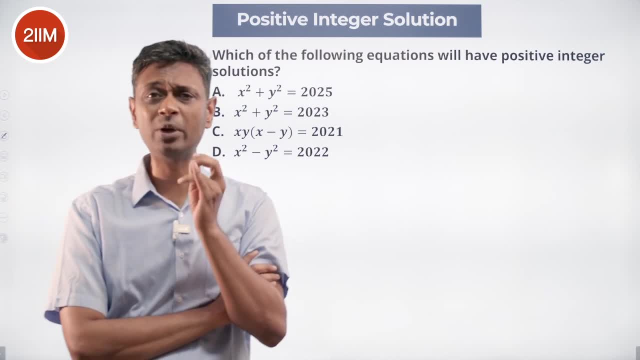 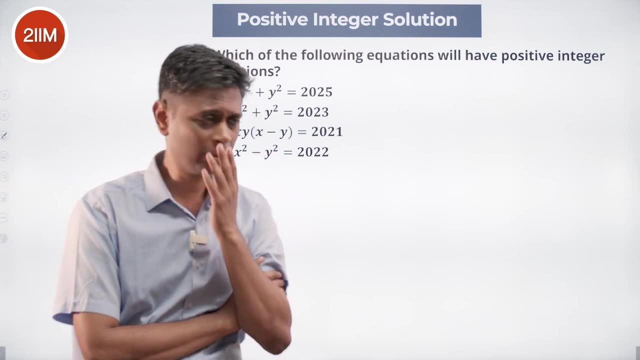 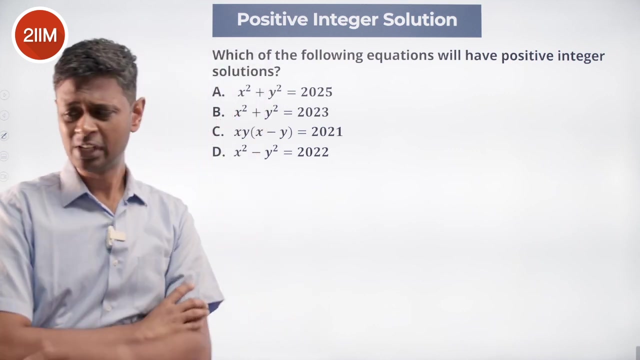 equal to 2025.. How are we going to even verify this? How am I going to find out whether there are possible integer solutions to this? How are we going to figure that out? How is that going to happen? 2025 is 45 square, which is useful, and we know that is useful. 2025 is 45 square, It is. 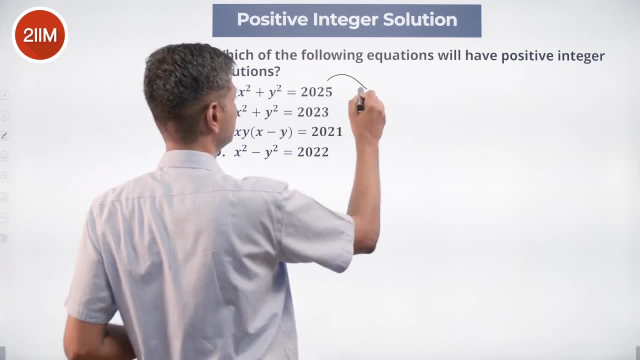 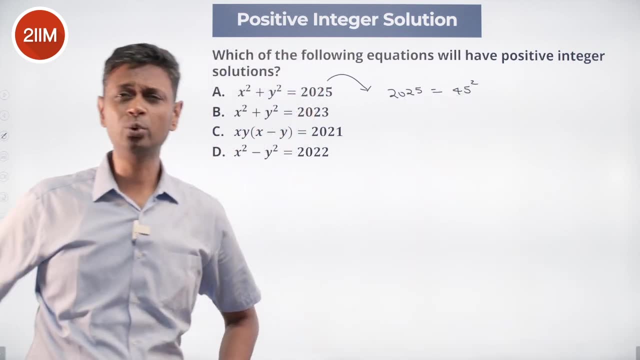 very nice to see if we can factorize this: 2025 is 45 square In my mind. once I knew that 2025 is 45 square, I have already done this question. This can work. Why So? because this number. 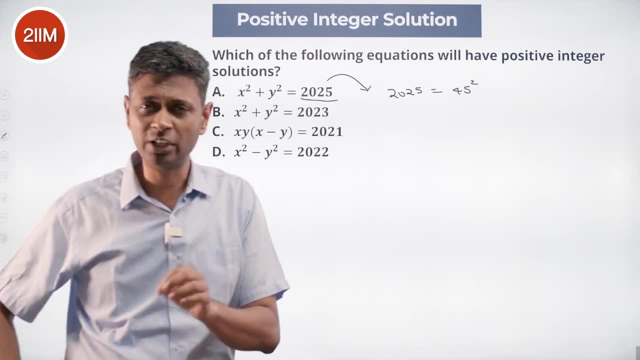 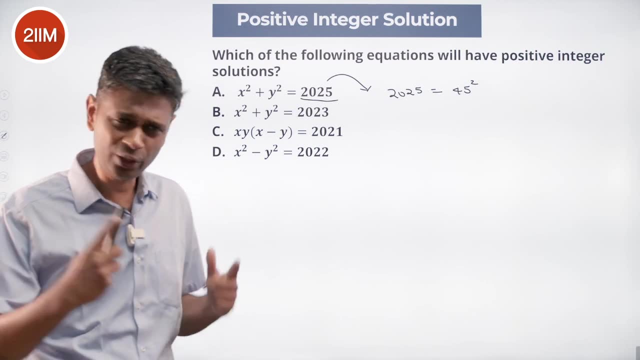 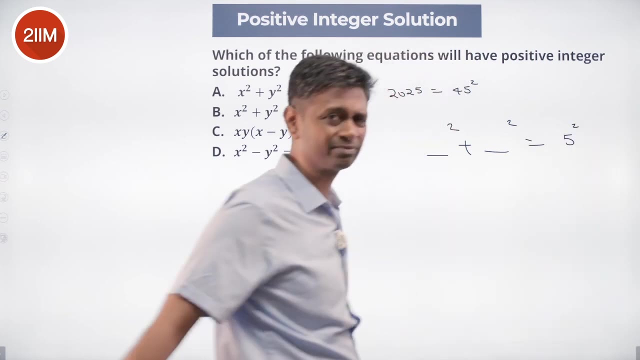 is 45 square. 45 is 5 into 9.. This number is multiple of 5 square. So I already know something square plus something square equals 5 square. I know that It is a very famous Pythagorean triplet. I know that 3 square. 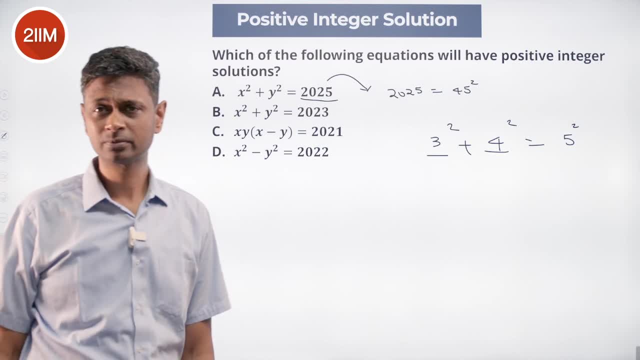 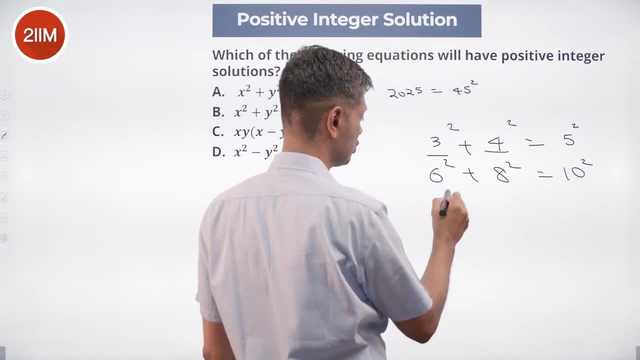 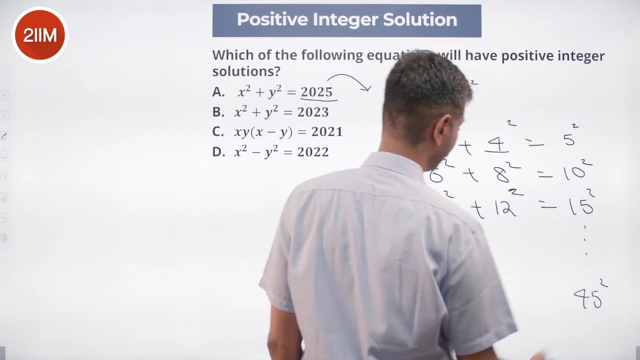 plus 4 square is equal to 5 square. Therefore, I know that 6 square plus 8 square equal to 10 square. I know that 9 square plus 12 square equals 15 square. plus 45 square, 27 square. 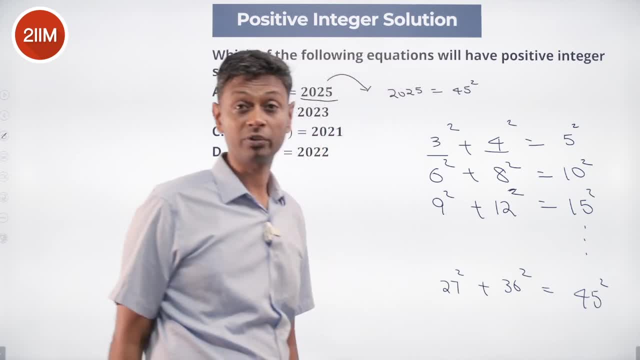 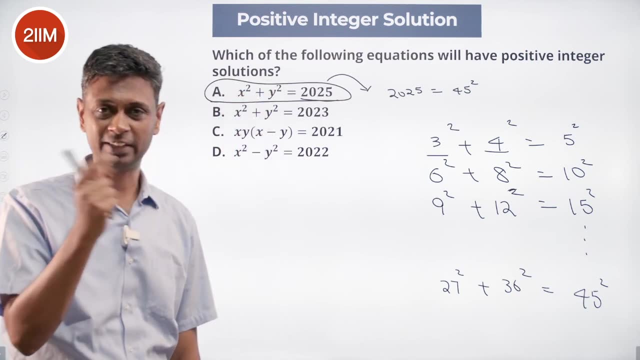 plus 36 square should be equal to 45 square. I already know straight away that this appears to be possible. I am not happy. I am not going to stop with that. I am not going to say, hey, done, I do not need to look any further. I will have to carve open the other things as well. 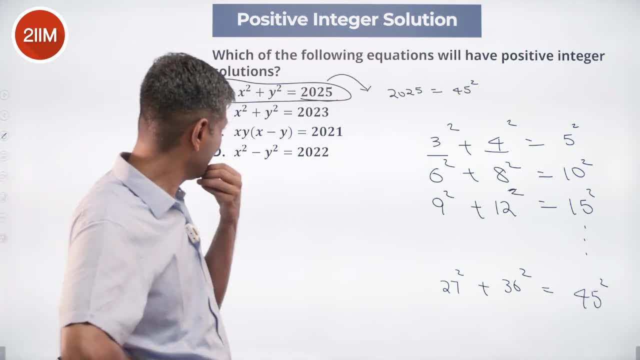 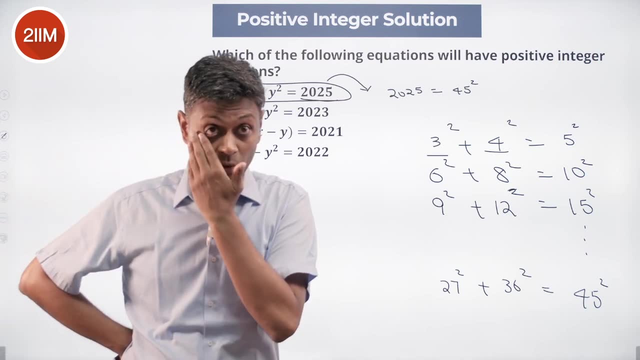 2023, 2023, is that possible? Can that happen? xy into x minus y is 2021.. x square minus y square is 2022.. But I know that the first one is possible. I want to see if, by some chance. 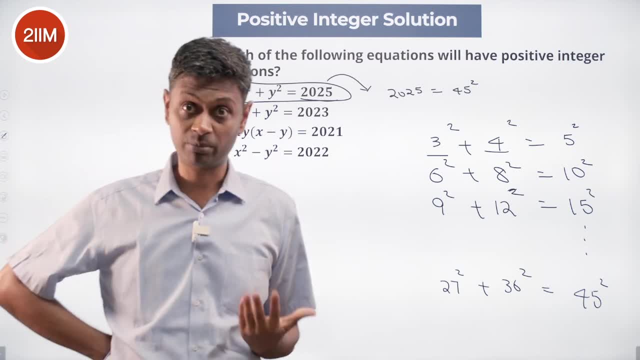 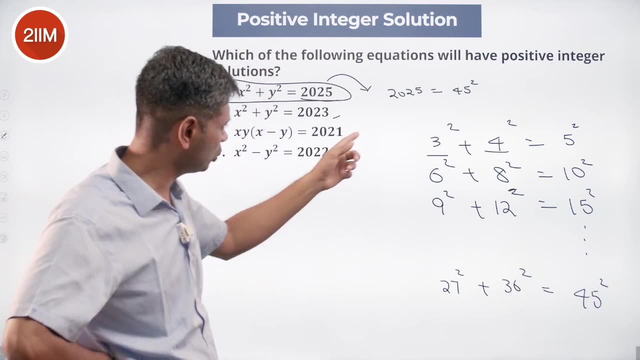 something else is possible, in which case I will have to revisit the first one. Maybe I have done some mistake. I want to prove that the others are not possible. When I look at this, 2023 and 2021 are weird numbers And there is a x square plus y square. 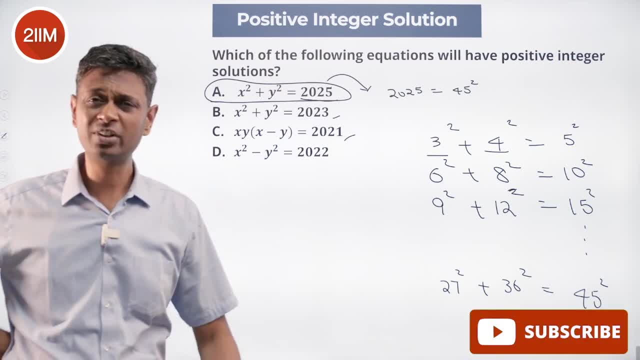 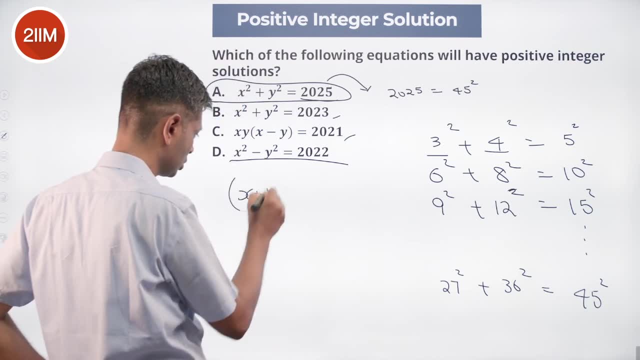 which I cannot say. I cannot say that it is possible. I cannot say that it is possible, I cannot factorize really. But then x square minus y square here, straight away, I am thinking this fellow, I can just factorize and get it done. This is x plus y into x minus y, which is 2022.. 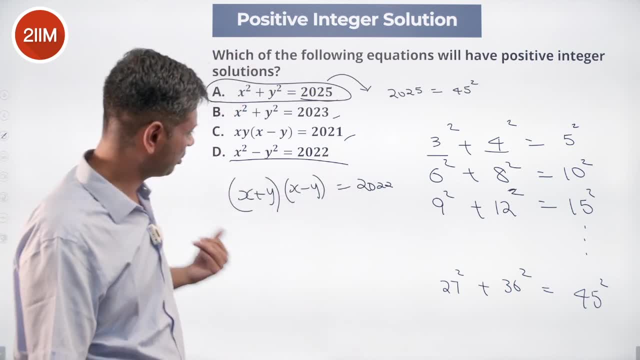 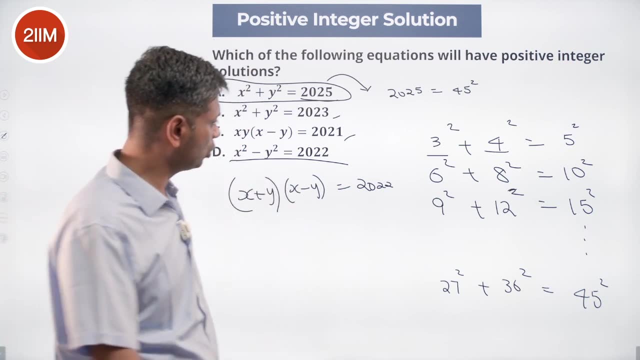 That means, if I break 2022 in two parts, put one of them as x plus y, put one of them as x minus y, I should be able to solve it and get x and y. Why is it not happening? So 2022 is 20 into 101.. 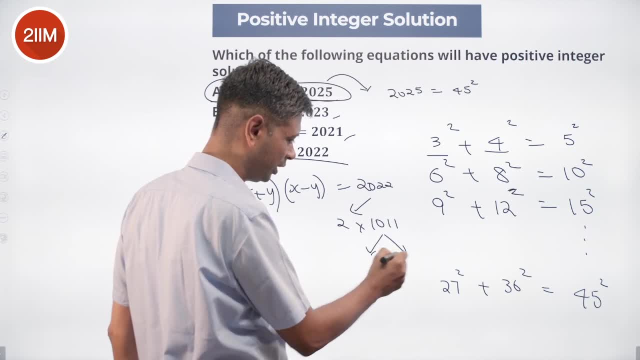 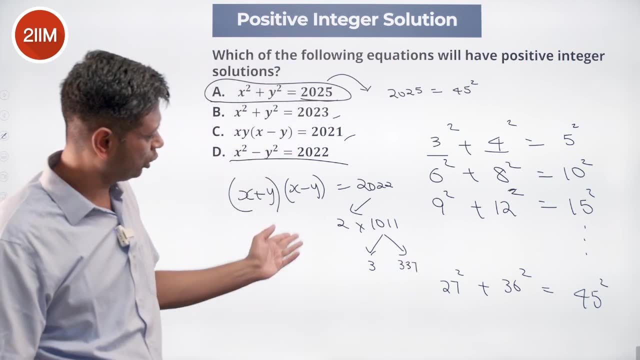 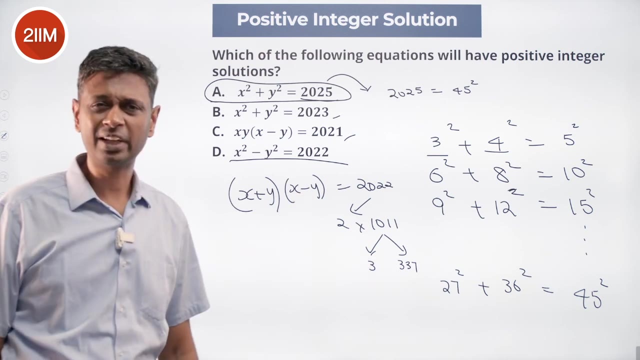 In 1011, it is a multiple of 3.. 3 into 337.. So it could be 2 into 1011, 3 into 774, 6 into 337.. I can write in all these forms x plus y into x minus y, which means I should be able to solve. 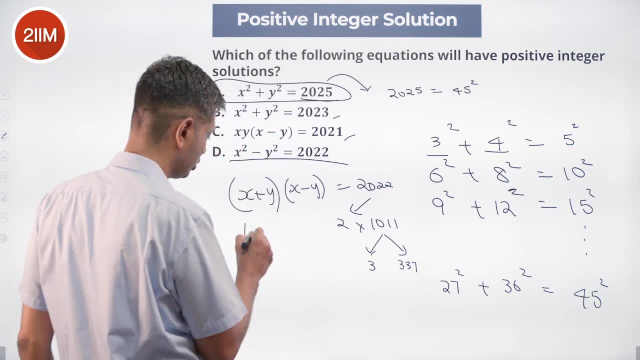 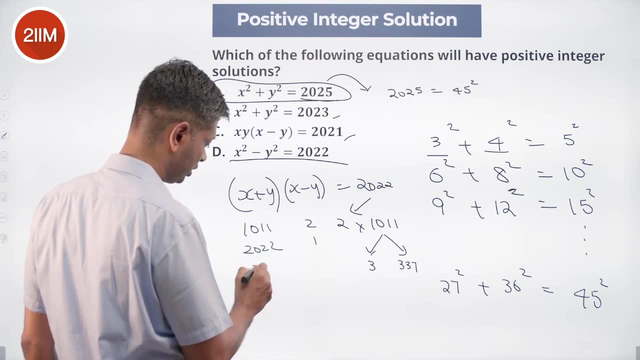 and get, Except. it is not possible, because if I put this as 1011, this is 2.. If I put this as 2022, this is 1.. If I put this as 337, this is 6.. What beautifully happens? very, very interesting idea. 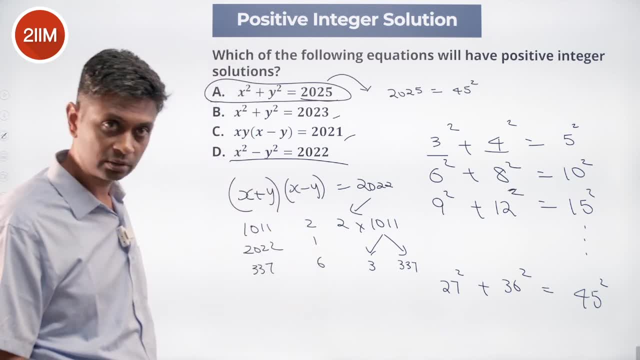 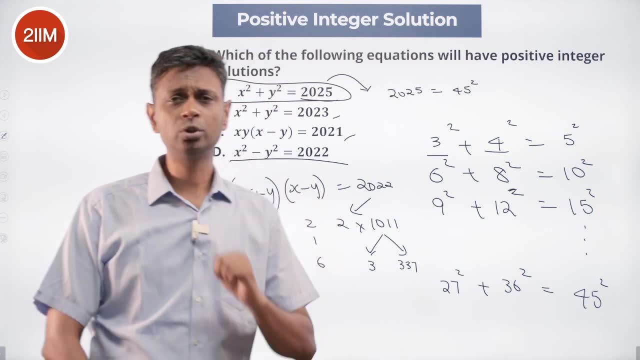 I have an odd number and an even number, Even number and an odd number, Odd number and even number. 2022 is a multiple of 2, but not a multiple of 4.. So 2022, if I factorize it. 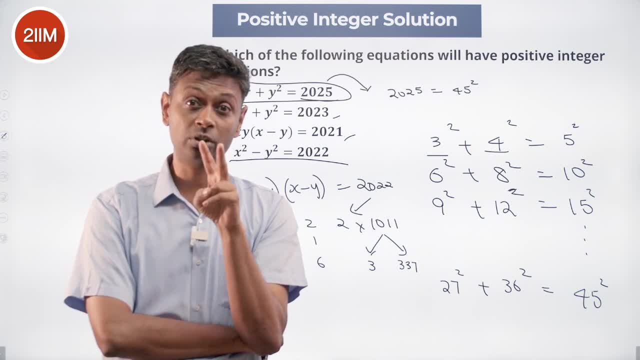 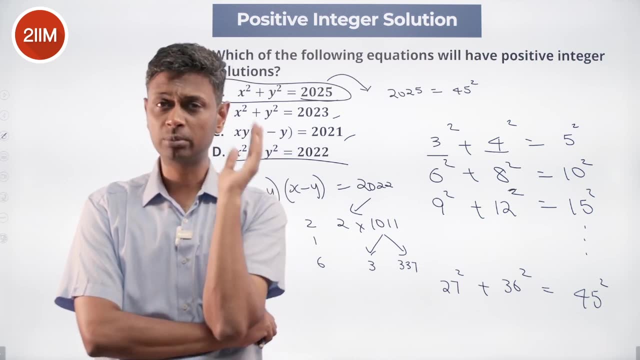 I cannot write it as a product of two odd numbers. I cannot write it as a product of two even numbers. It will have to be one odd number into one even number. One of the two numbers has to be even and only one of the two numbers can be even, Which is a problem. 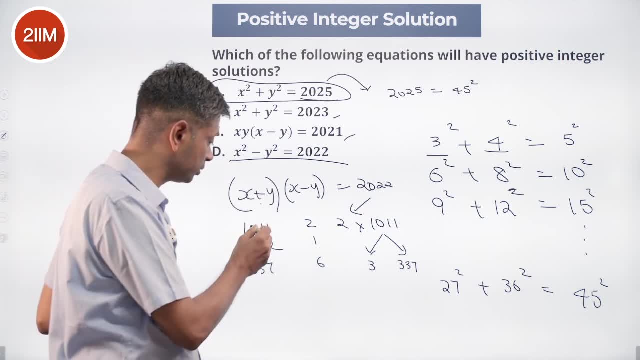 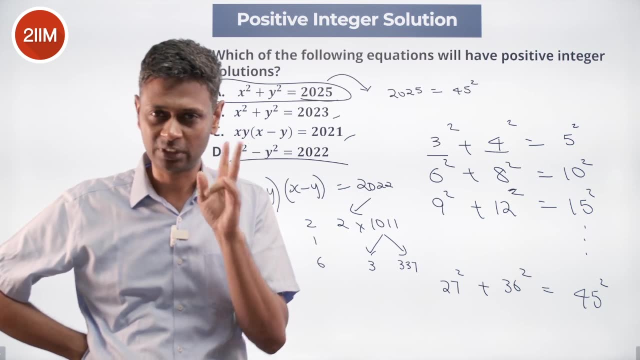 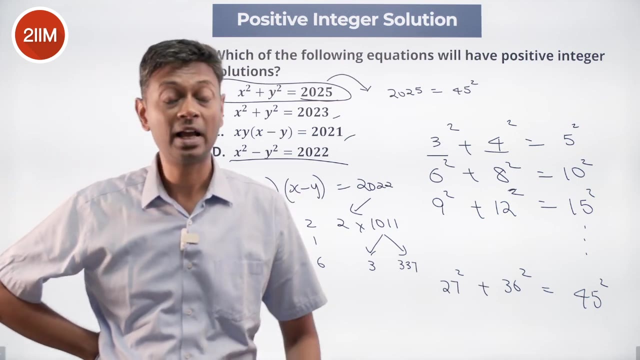 because, if you think about it, if sum of two numbers is odd, sum of two natural numbers is odd, then one of them has to be odd, other has to be even. That means the difference also has to be odd. I cannot have a mechanism where sum of two natural numbers is odd and their 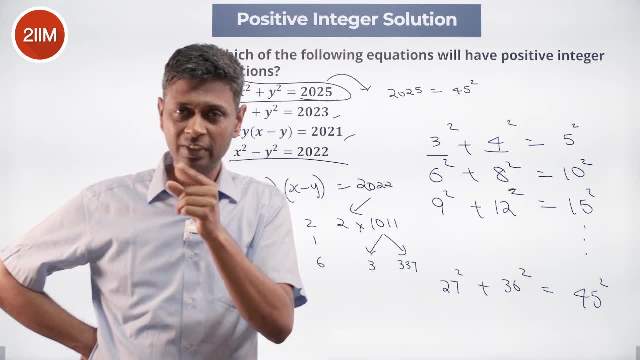 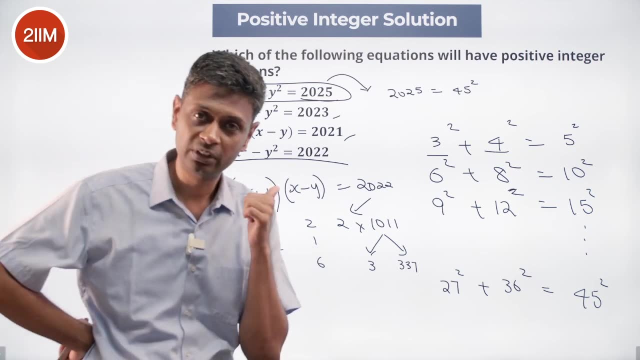 difference is. even The difference between two natural numbers is even. So if I factorize even, either both are odd or both are. even If the difference is even, sum should also be. even if the sum is even, difference should also be. even if sum of two natural numbers is odd, different should also be. 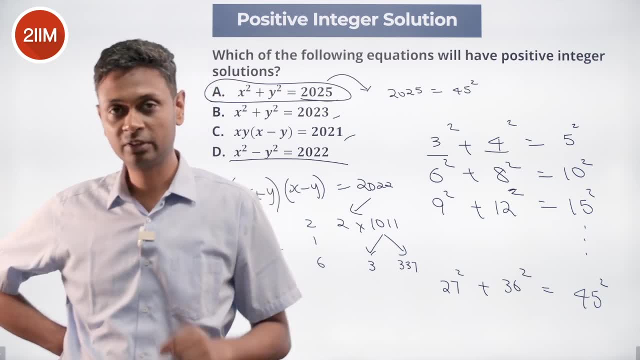 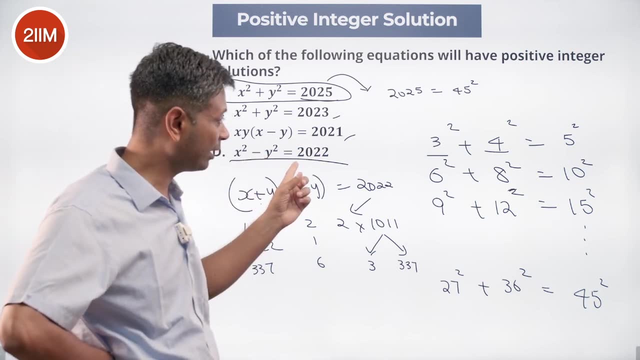 odd. if sum of two natural numbers is even different, should also be even. So if I have x2-y2, this can be equal to. x2-y2 can be equal to an odd number. x plus y, x minus y. both are odd. that is possible. 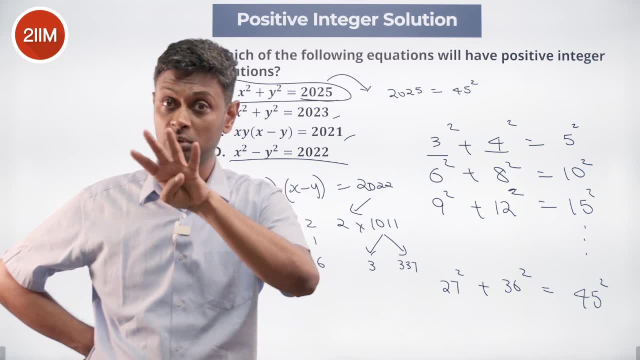 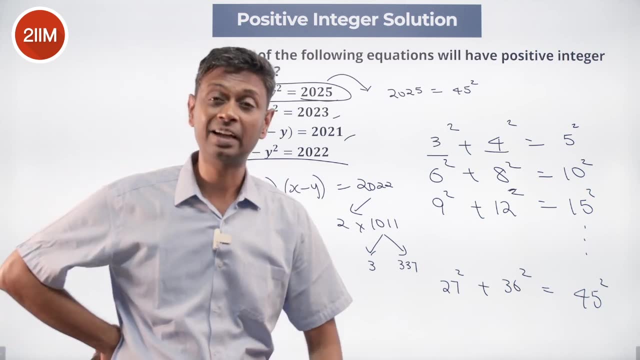 It can be equal to an even number, in which case the even number should be a multiple of 4.. Both parts, x plus y and x minus y, should be even. I cannot have x square minus y square equal to an even number that contains only a 2, not a 4.. 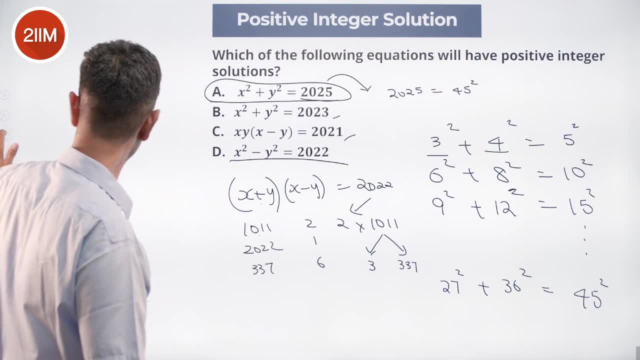 Therefore, this is not possible. So by far the most tempting choice. Look at this and say, look, I can write this: x plus y and x minus y, I am through. And then I can simplify: no, except we are not through. 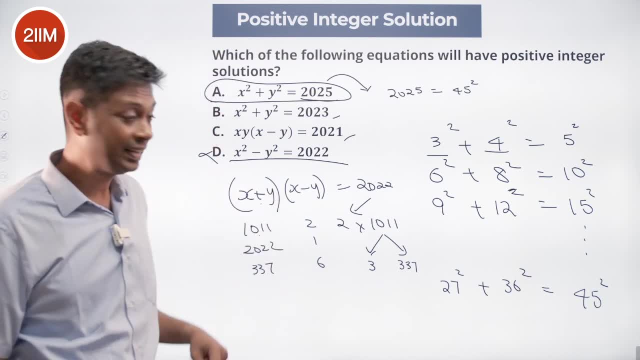 We solve: x plus y equal to 1,, 0,, 1,, 1,. x minus y equal to 2.. Then 2x will be 1, 0,, 1, 3, x will be 1, 0,, 1, 3 by 2,, no longer an integer, no longer a natural number. 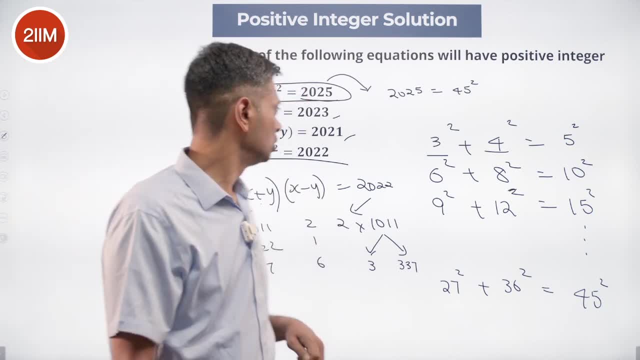 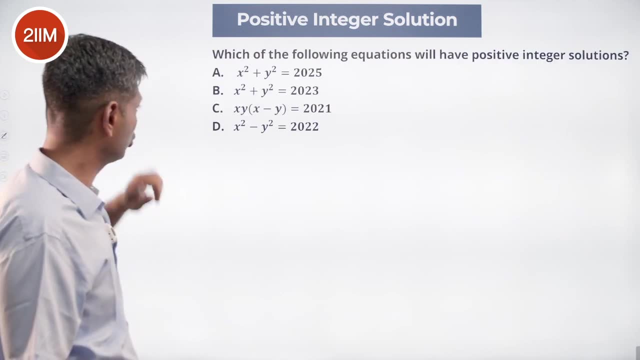 Because since it says positive integer solutions, it does not work. Okay, super, so this does not work. These two I still have to worry about, Fine xy into x minus y is 2, 0, 2, 1.. 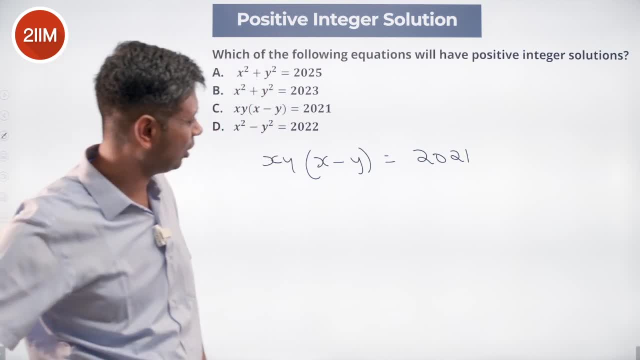 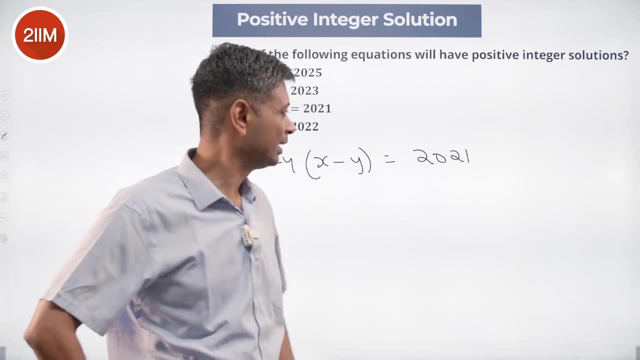 2, 0,. 2, 1 is one of those annoying numbers, So not Not a multiple of 2,, not a multiple of 3, not a multiple of 5, not a multiple of 7.. 21 is a multiple of 7, 2000 is not a multiple of 7, not a multiple of 11.. 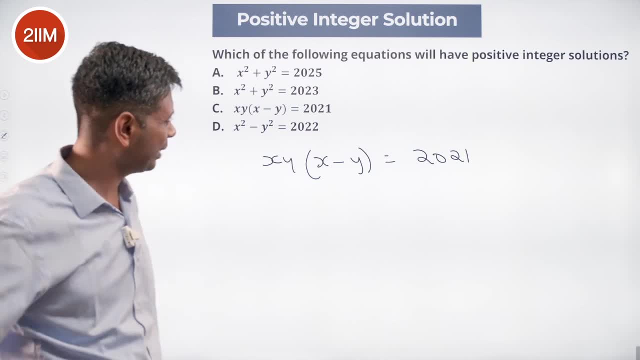 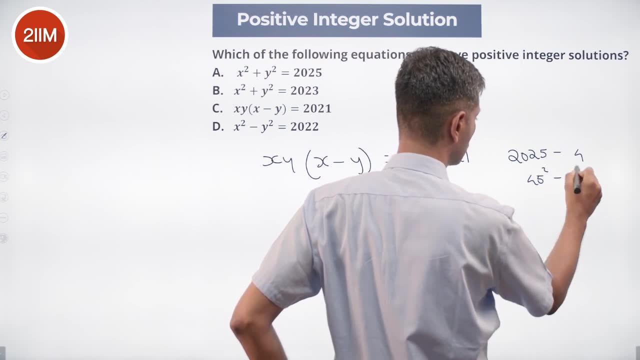 I will have to check for 13,, 17,, 19,. all of that Except. we can think of this as 2, 0,, 2, 5 minus 4, 45 square minus 2, square 45 plus 2 into 45 minus 2.. 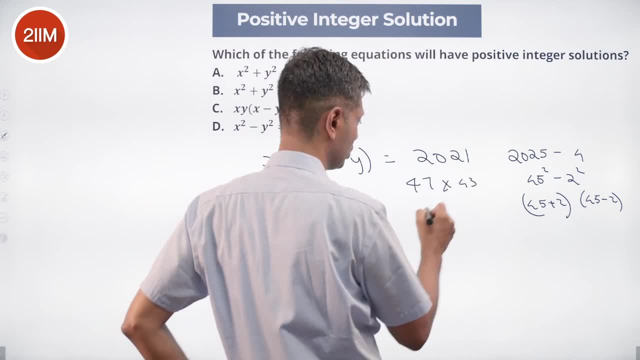 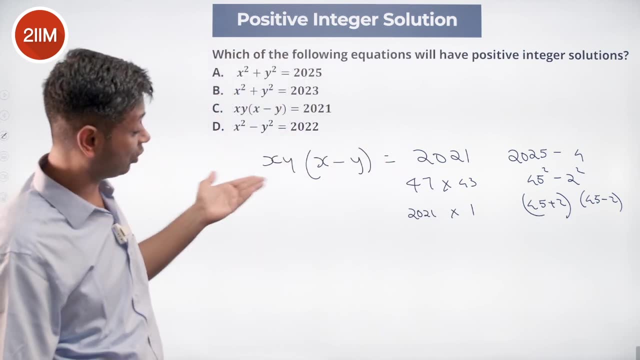 This can be written as 47 into 43. Or 2, 0,, 2, 1 into 1.. One of these two has to be this: If I put x into y is 47, x and y can be only 1 and 47.. 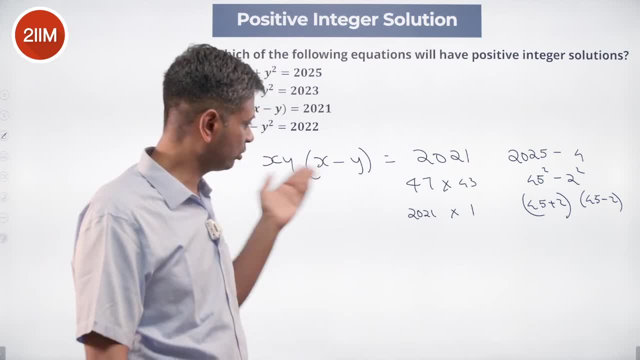 x minus y cannot be 43, out. If I put x into y is 2, 0,, 2, 1, then I have 47 into 43, or 2, 0,, 2, 1 into 1.. 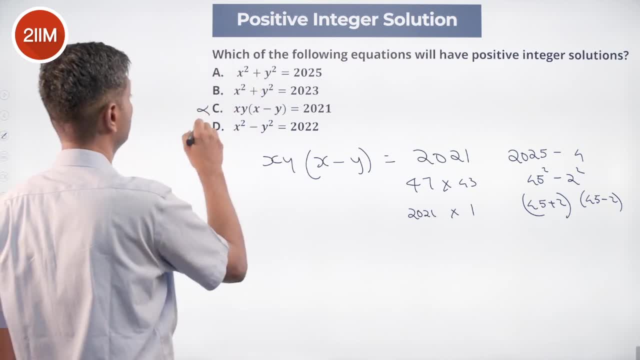 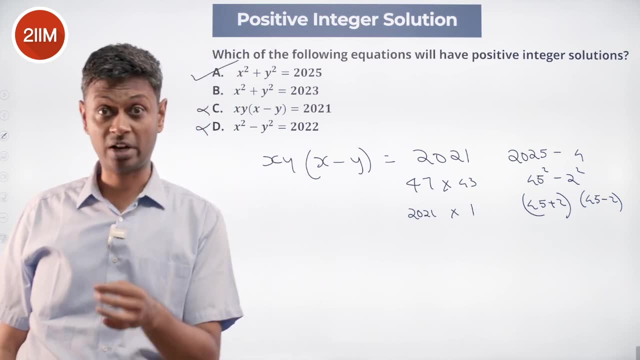 x minus y doesn't work. Therefore, this: there are no solutions. this, there are no solutions. this, there is a solution, And so I have kind of gotten to the idea that the first one stands out very happy. It is just 3,, 4,, 5 into something. 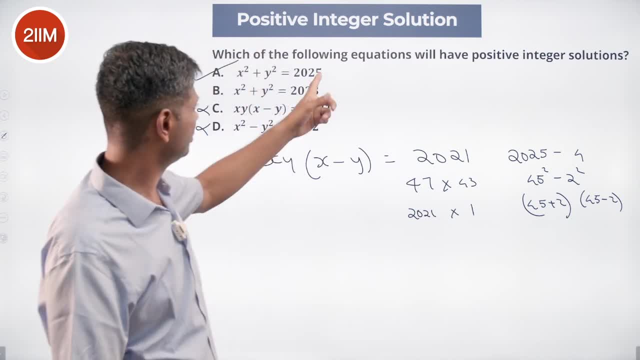 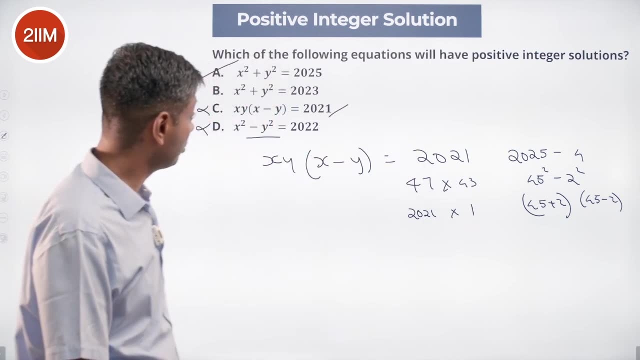 I am super happy with that because I understand Pythagorean triplets. So this is good. I have kind of established that this is not possible at all. this is not possible at all. Two things have gone my way. Now let me see if I can prove that this is not possible at all. 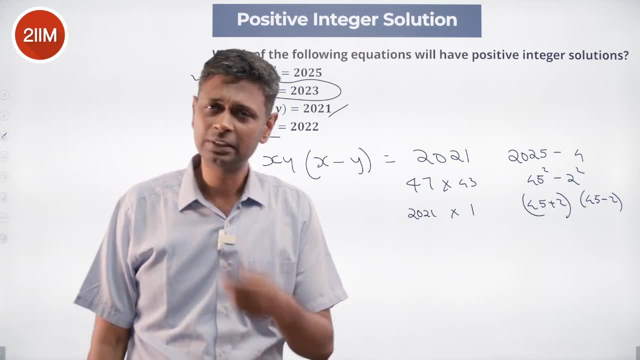 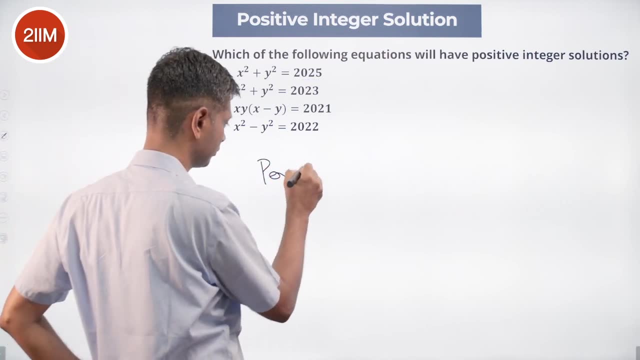 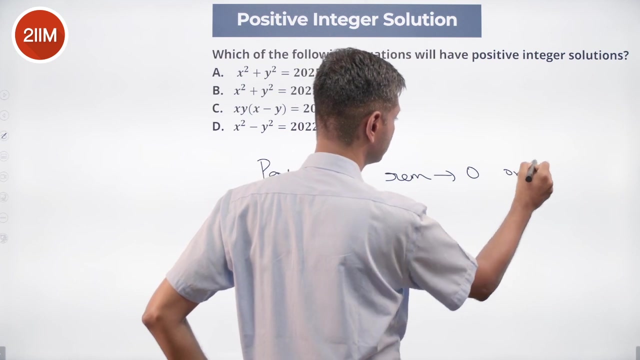 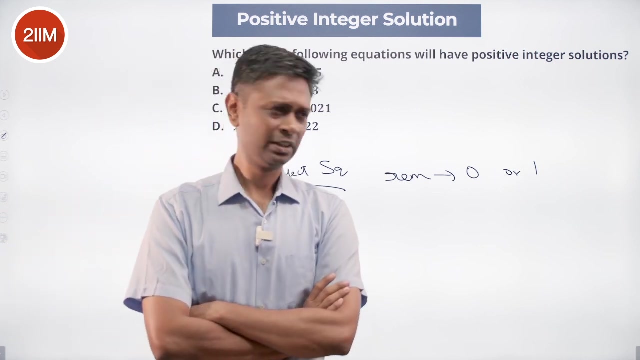 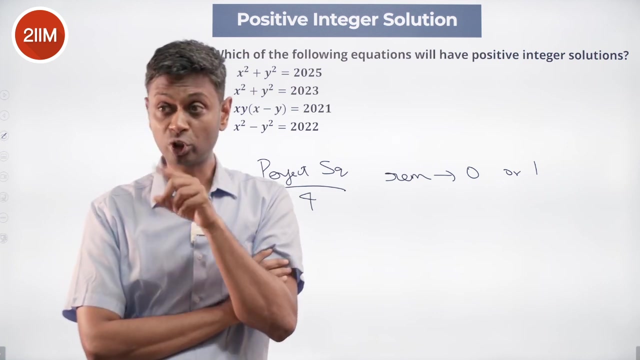 x square plus y square equals 2023.. It is tricky. I am going to use any perfect square. So I am going to use any perfect square divided by 4, remainder will be either 0 or 1,. any perfect square divided by 4, the remainder will be either 0 or 1, remainder cannot be 2 or 3,. why can it not be 2, divide the number by 4,. if it is a multiple of, if its remainder is 2,, then that means the number has a 2 in it, but only one 2 in it. a perfect square cannot have only one 2,. that is what it looks. 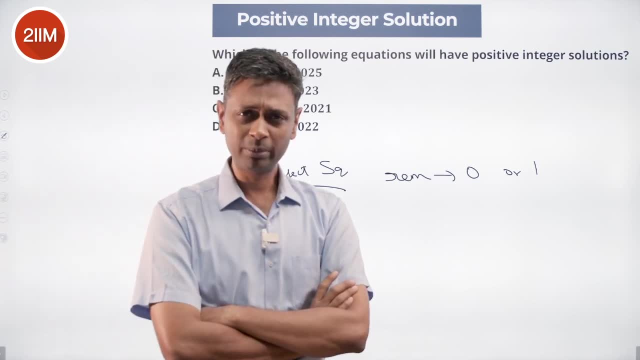 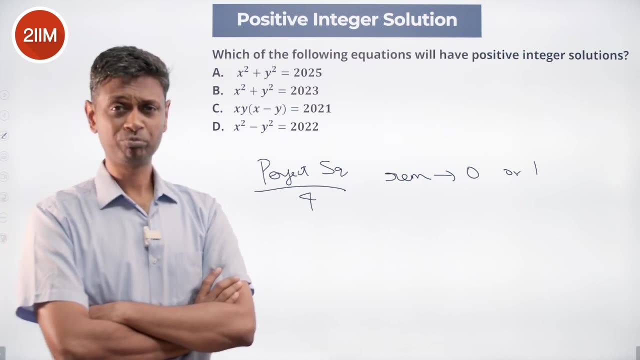 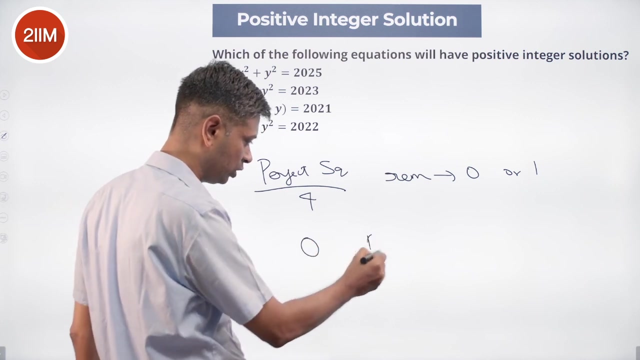 So it cannot. the remainder cannot be 2, the remainder cannot be 3.. Either perfect square divided by 4, remainder is either 0 or 1, if you know that, then it is super easy to simplify why: because I have two perfect squares. they could either have remainder 0 and 0, 0 and 1, or 1 and 1,, 1 and 0, again, not worrying about the order. 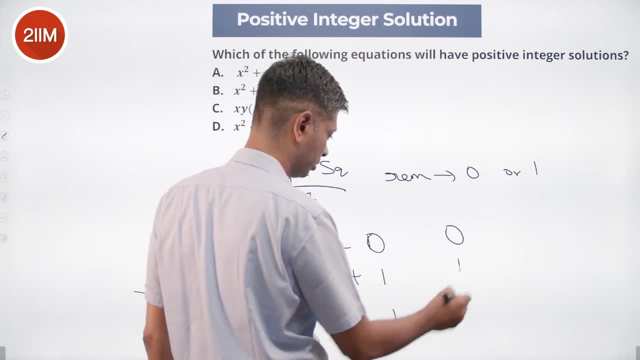 If it is 0 plus 0, remainder will be 0, 0 plus 1, remainder will be 1, 1 plus 1, remainder will be 2, 2023 divided by 4, remainder is 3, that cannot be sum of 2.. 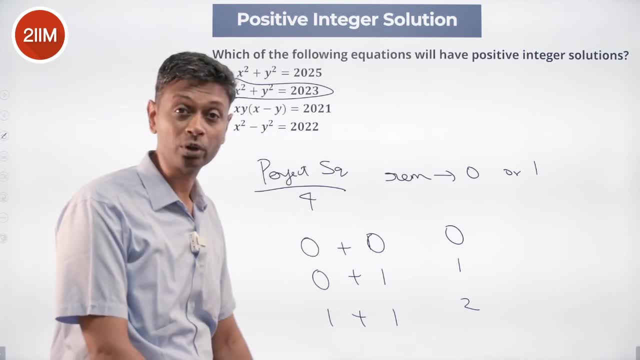 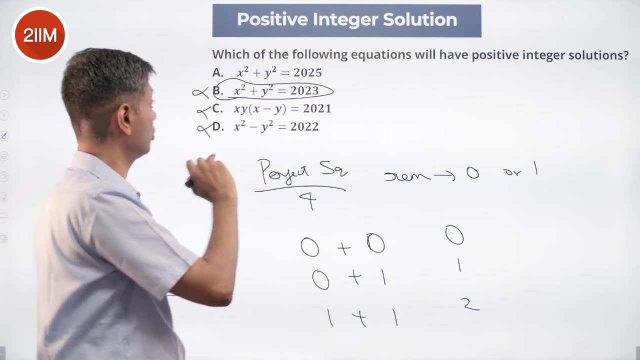 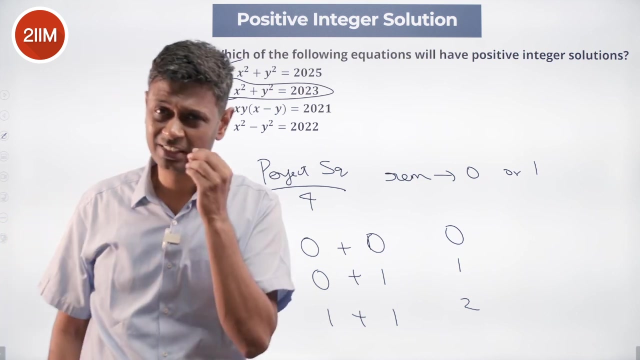 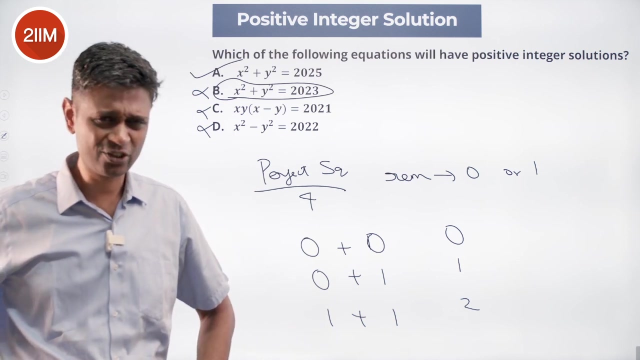 So we have two perfect squares. we can rule that out. that is the more rigorous way of establishing that. hey, this is not possible. these two are easily established. these two are not possible. this is definitely possible. Again, from an exam point of view or solving point of view. you can just sense that 2, 0, 2, 5 is a perfect square. it is a multiple of 5 whole square, that is 45 square, or 9 square into 5 square. 3, 4, 5 is a Pythagorean triplet: 3 into 9,, 4 into 9,, 5 into 9,. 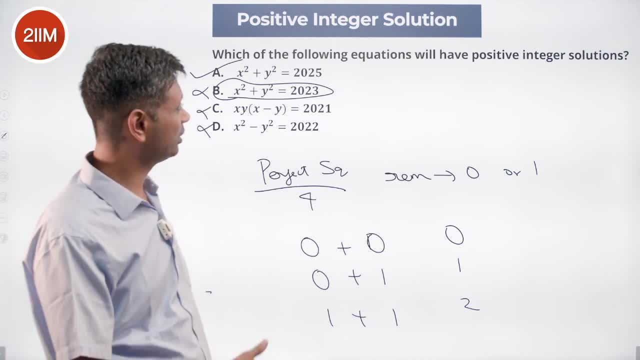 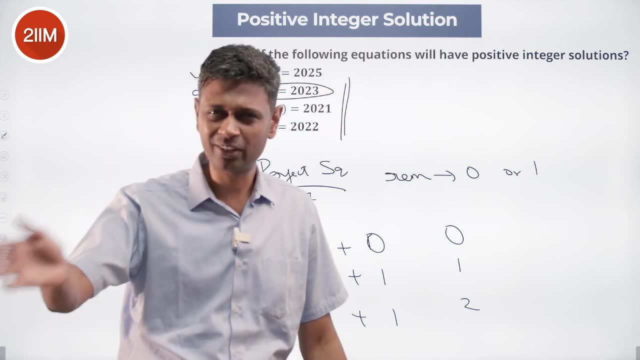 will also be a Pythagorean interpret and I've got one solution. all I need to do is that does have positive integer solutions. I'm through and then I have to establish that these three do not have integer solutions, which I can later figure out, so you can know that.